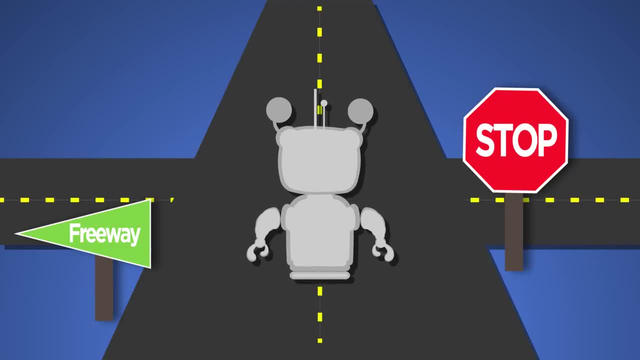 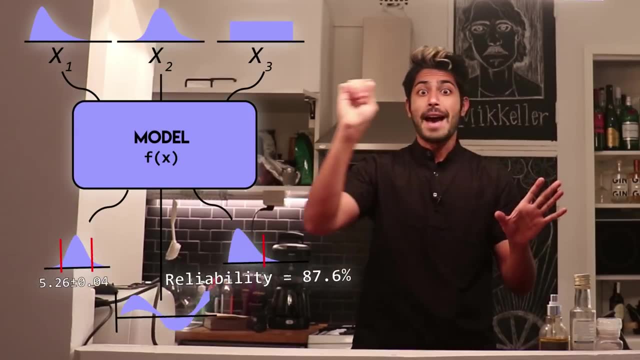 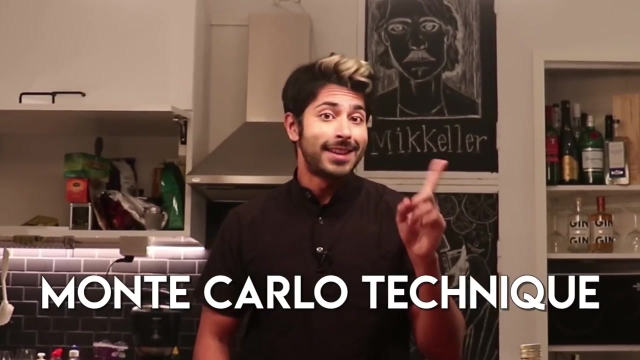 without building a model, And this is called model-free learning. Model-free learning involves predicting the value function of a certain policy without having a concrete model of the environment. The simplest way to do this is using the Monte Carlo technique, meaning using repeated random. 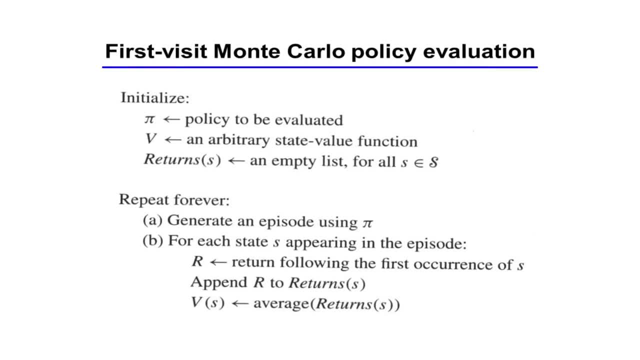 sampling to obtain numerical results. But this only works on episodic tasks where you have a certain set of actions. then the episode ends with some total reward. Monte Carlo learning states that the return of a state is just the mean average of the total reward from when a state appeared onwards. 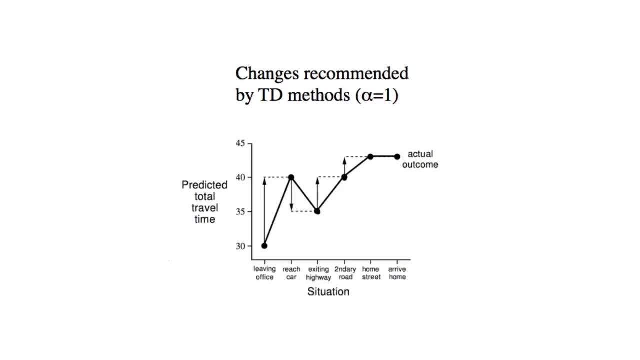 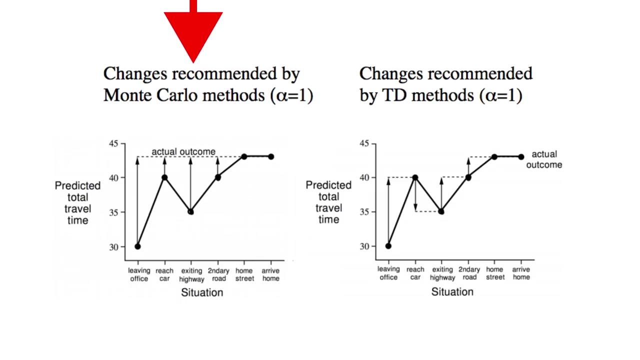 So, in order to reduce the variance, we can use a different method of prediction. Temporal difference learning updates the values of each state based on a prediction of the final return. For example, let's say Monte Carlo learning takes 100 actions and then updates them all. 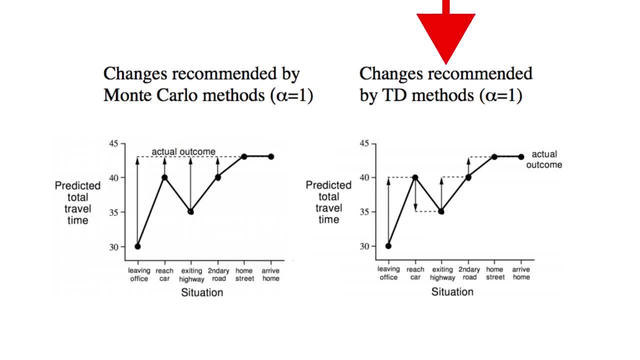 based on the final return. Td learning. Td learning would take an action and then update the value of the previous action based on the value of the current action. Td learning has the advantage of updating values on more recent trends in order to capture. 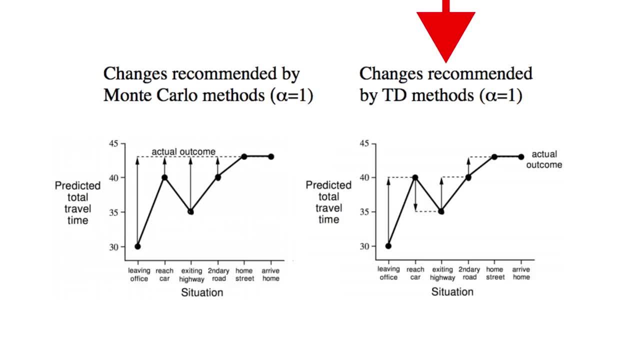 more of the effect of a certain state. Td has a lower variance than Monte Carlo, as each update depends on less factors. However, Monte Carlo has no bias, as values are updated directly towards the final return, while Td has some bias, as values are updated towards a prediction. 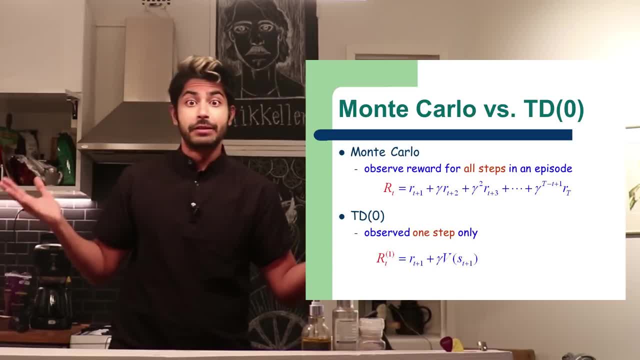 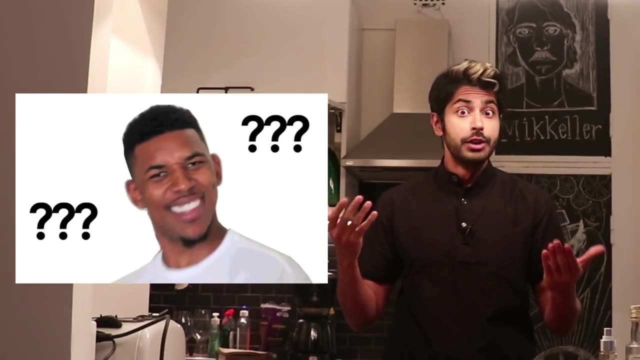 Both Td and Monte Carlo are actually opposite ends of a spectrum between full look ahead and one step look ahead. Any number of steps can be taken before passing the return back to an action, So a question arises: how many steps is optimal to look ahead? 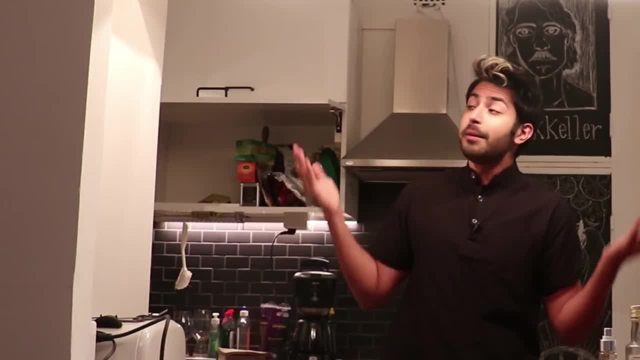 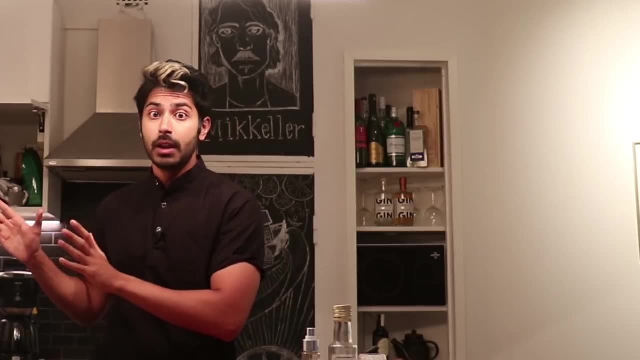 Well, it varies greatly depending on the environment, and it's often a hard-coded hyperparameter. Td learning, Td learning: A lot of people learn both the value function and the q function. What's that you said? Does Q stand for quick time? 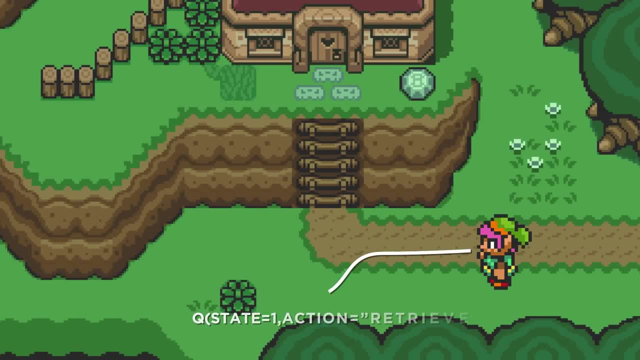 No, thankfully. If we want our AI to always choose an action that maximizes the discounted future reward, we'd want to use some form of Td learning. We could define a function q that represents the maximum discounted future reward when we perform an action A in state s and continue optimally from that point on. 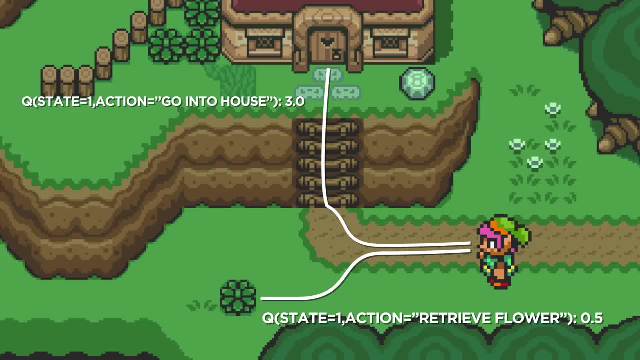 The way to think about this function is that it's the best possible score at the end of the game after performing an action A in a state S. It's called a Q function because it represents the quality of a certain action in a given state. 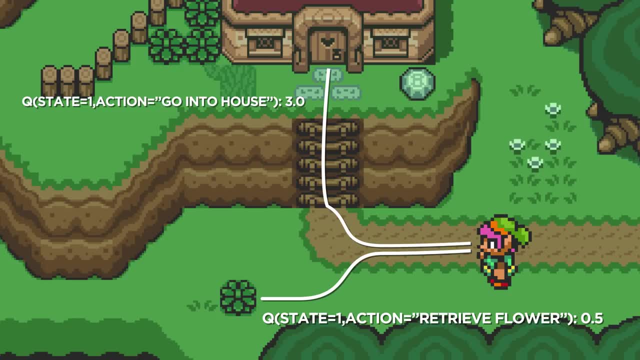 Using it, we can estimate the score at the end of the game knowing just the current state and action and not knowing actions and rewards coming after that. So suppose we're in a state and deciding whether we should take action A or B. We want to select the action that results in the highest score at the end of the game. 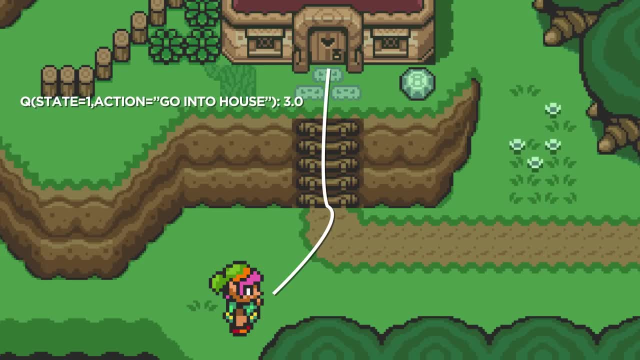 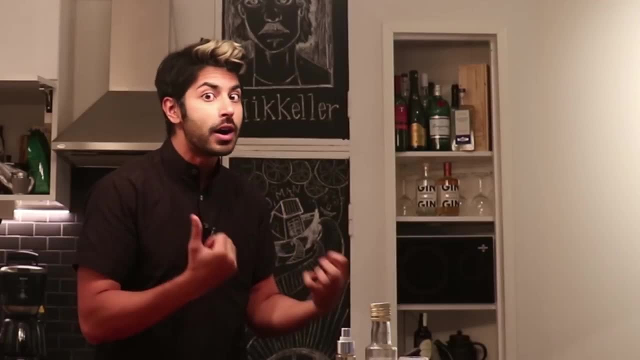 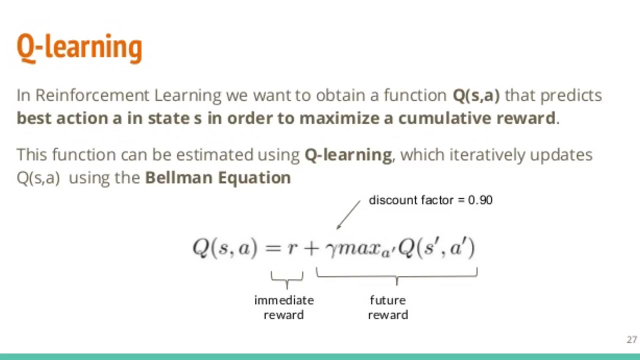 Once we have the magical Q function, the answer becomes really simple. We can just pick the action with the highest Q value. So we need to learn this Q function and we can call this process Q learning. We can express the Q value of state S and action A in terms of the Q value of the next state S. 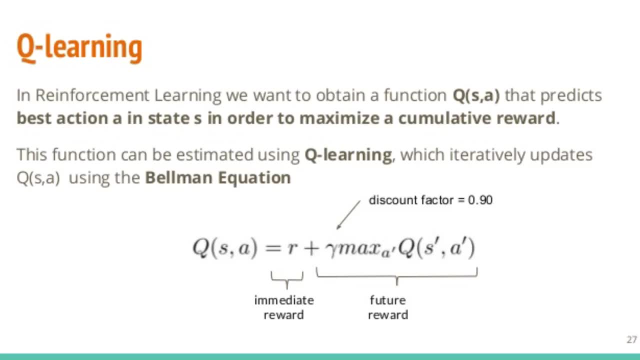 This is called the Bellman equation. If you think about it, it makes sense: Maximum future reward for the state and action is the immediate reward plus maximum future reward for the next state. The main idea in Q learning is that we can iteratively approximate the Q function using the Bellman equation. 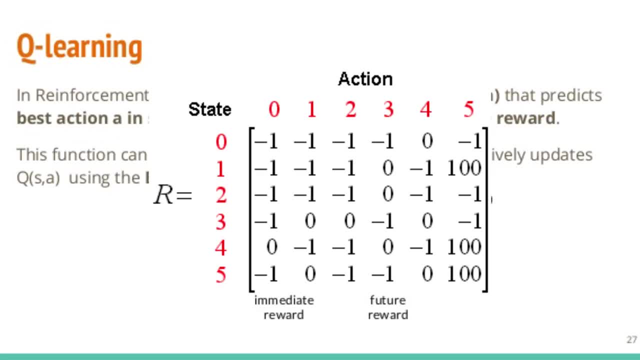 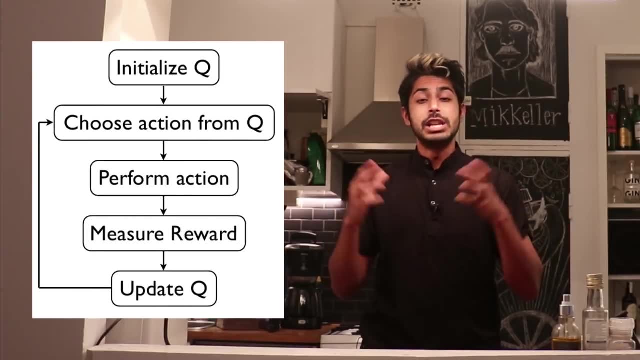 In the simplest case, the Q function is implemented as a table, with states as rows and actions as columns. So, to start, the Q table is initialized randomly, Then the agent starts to interact with the environment and upon each interaction the agent will observe the reward of its action and the state transition. 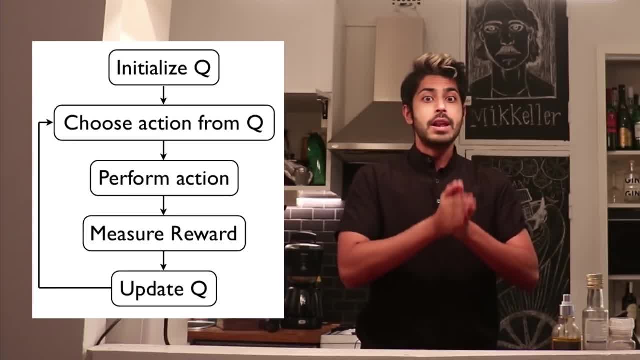 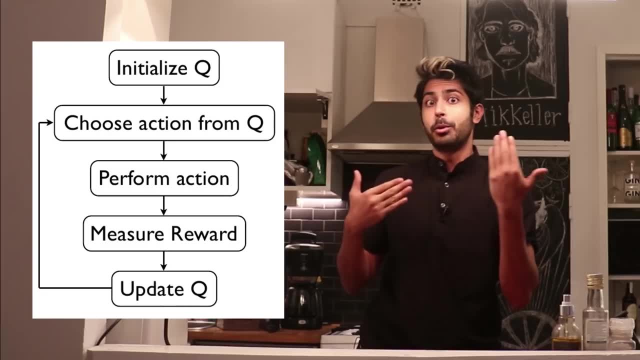 The agent computes the observed Q value and then updates its own estimate of Q. So we've got a basic iteration going and it works for simple policies. However, there's a problem: It's not exploring like Hernan Cortes Shout out to AP History. 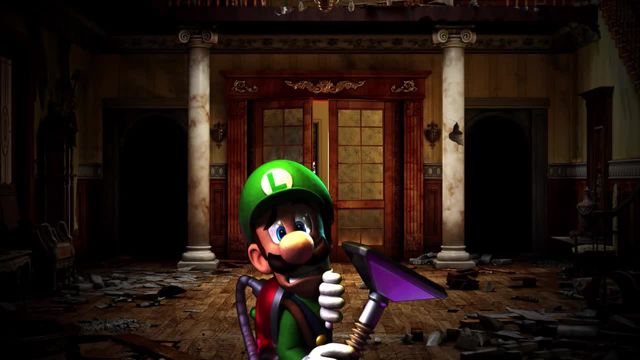 Let's say we're at a state with two doors. One door gives a reward of plus one every time and the other door gives zero reward but has a 10% chance of giving a 100 reward On the first run. the second door doesn't get lucky and returns a reward of zero. 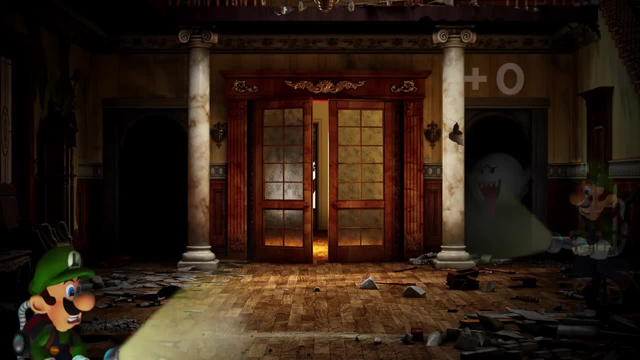 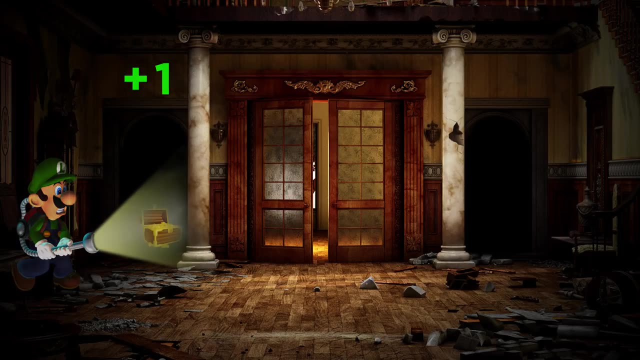 Since it's acting greedily. the AI will only ever take the first door, since it considers it the better option. So how do we fix this Random exploration? At some probability, the program will take a random action instead of taking the optimal action. 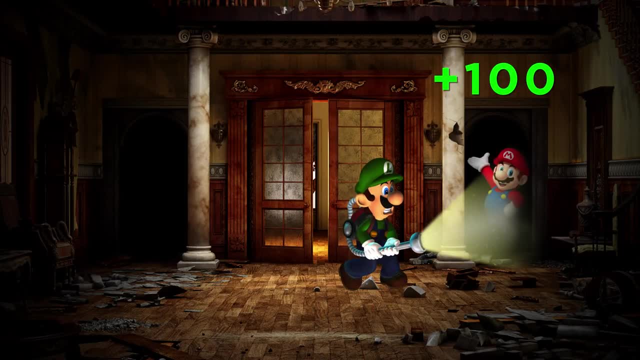 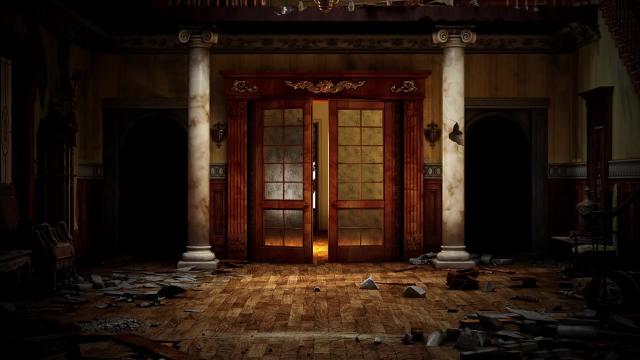 This allows it to eventually figure out that there is some extremely high reward hidden behind the second door if it tries it out. However, we want the AI to eventually converge at some optimal policy so we can lower the probability of taking a random action over time, as the agent becomes more confident with its estimate of Q values. 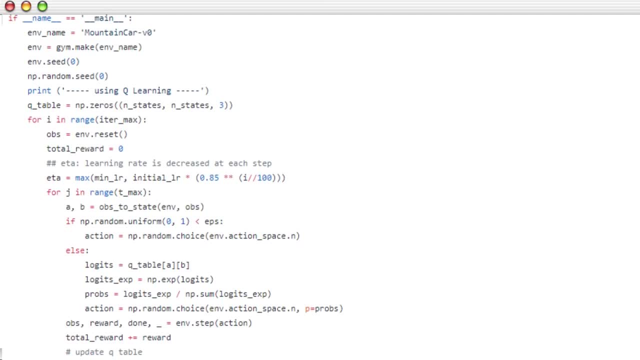 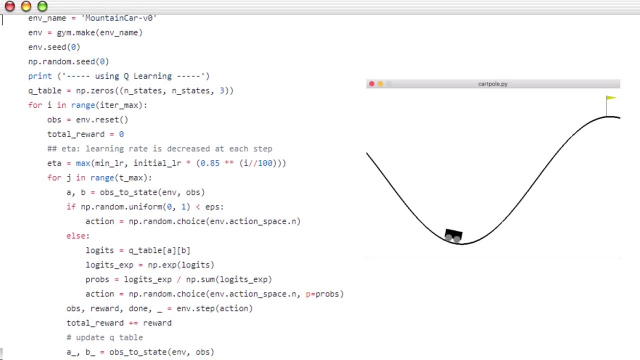 So, using Q learning and OpenAI's gym environment, we can teach a mountain car how to successfully climb a mountain. In this environment, there is a car on a one-dimensional track between two mountains. The goal of the car is to climb the mountain on its right. 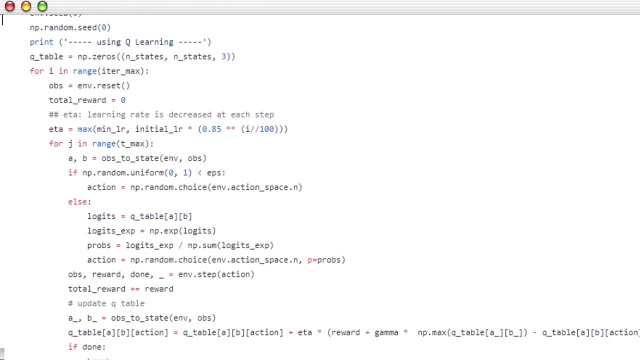 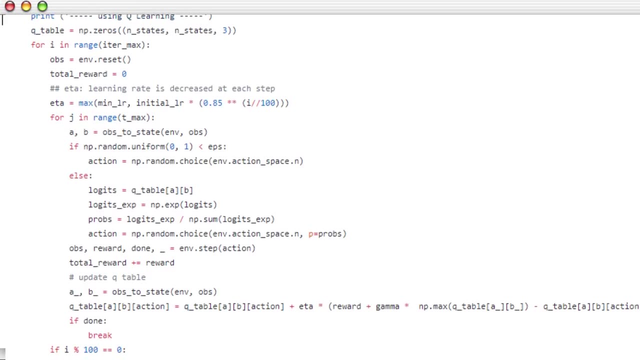 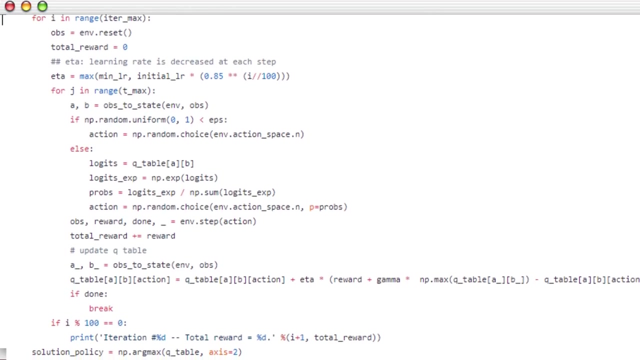 However, the engine is not strong enough to climb mountains without having to go back to gain some momentum by climbing the mountain on the left. Here the agent is the car and possible actions are: drive left, do nothing or drive right. At every time step, the agent receives a penalty of minus one. 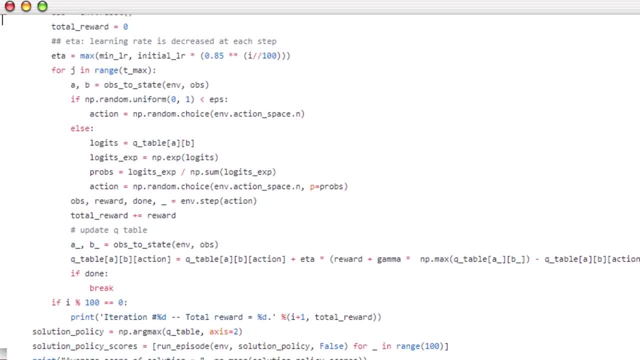 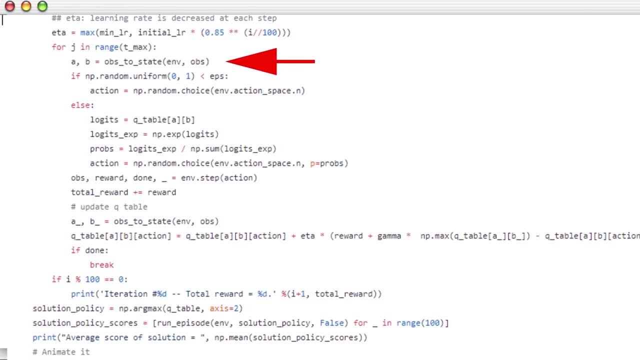 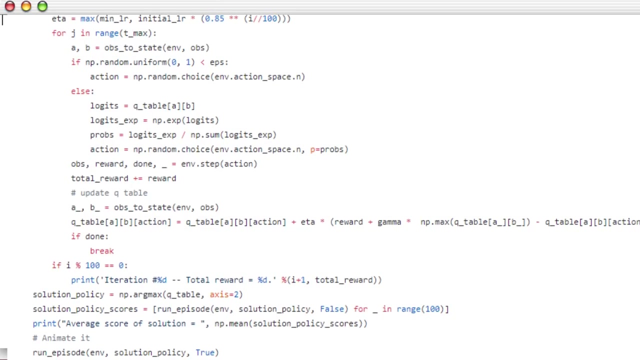 which means that the goal of the agent is to climb the right mountain as fast as possible to minimize the sum of negative one penalties it receives. The observation is two continuous variables representing the velocity and the position of the car. Since the observation variables are continuous for our algorithm, we discretize the observed values in order to use Q learning. 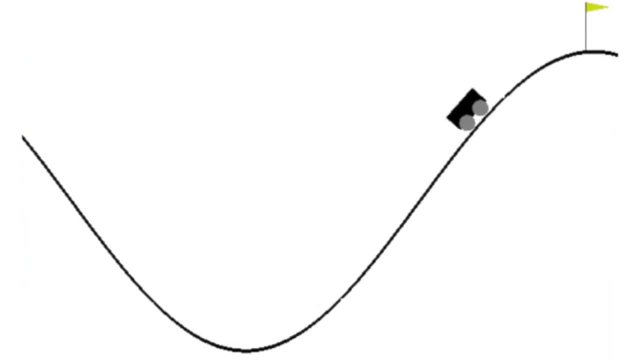 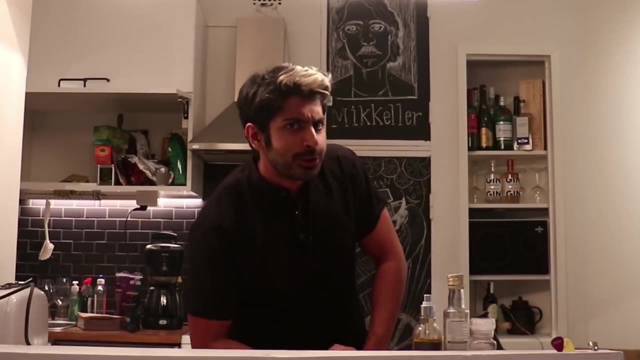 Initially, the car will take forever to climb if we select a random action, But after learning, it learns how to climb the mountain within less than a hundred time steps. You're still with me, right? Of course you are, you beautiful wizard.